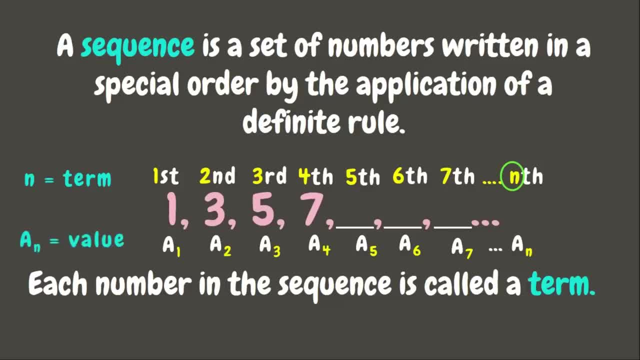 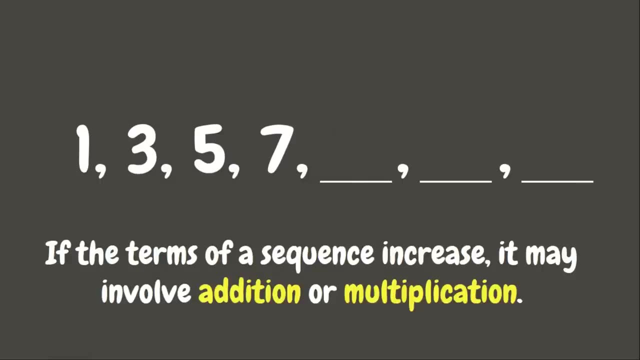 which is a sub n. this represents the value of each term. now that you already know what the sequence is, let us try to find out and solve for the next three numbers of this sequence. if the terms of the sequence increase, it may involve addition or multiplication. here we can see that the sequence increases. now what? 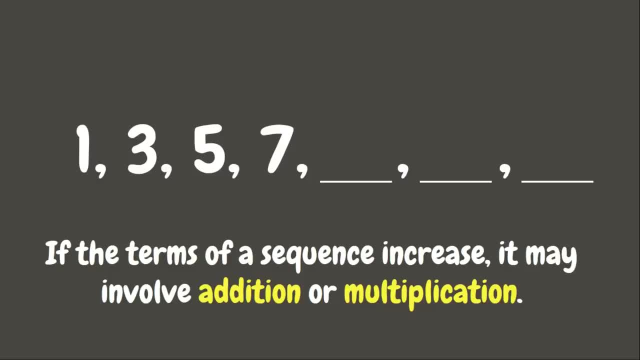 do you think what should we do to number one, which is the first term, to get the second term, which is three? great job, we need to add two. if we add two to our second term, which is three, we'll get five. next, five plus two is seven. 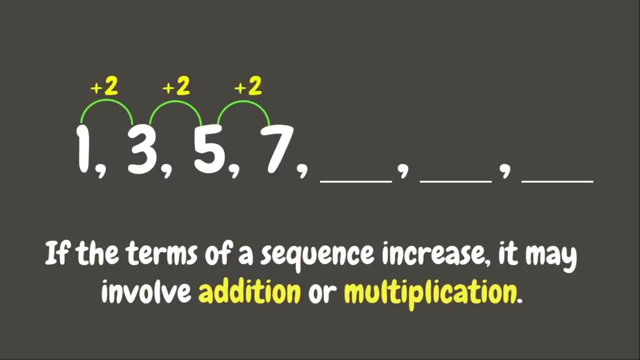 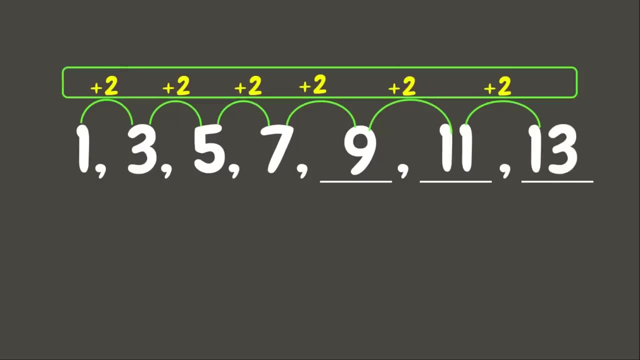 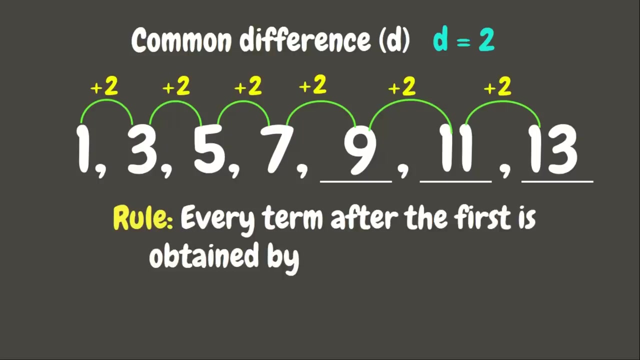 therefore, if we add two to seven, we'll get the next term, which is nine and nine, eleven and then thirteen. these numbers are what we call the common difference, which is represented by small letter D. this means that the common difference is two. here we can generate a general rule that, for every term after the first, is: 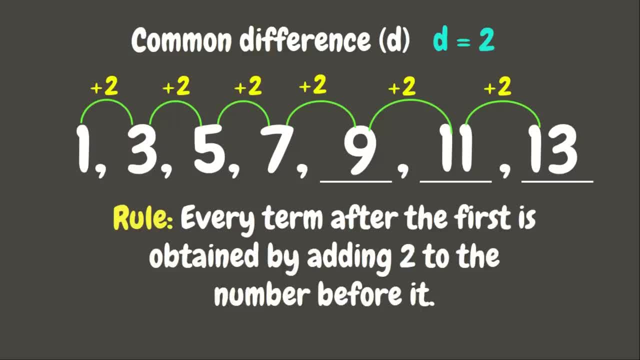 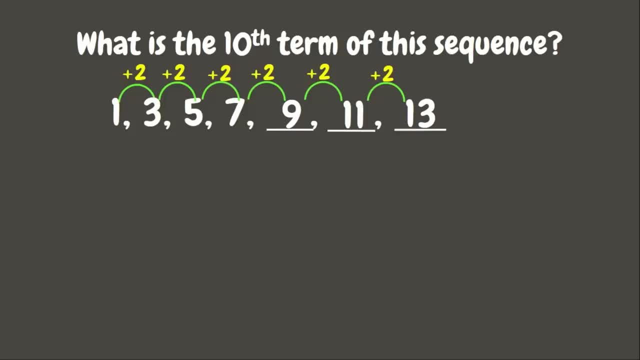 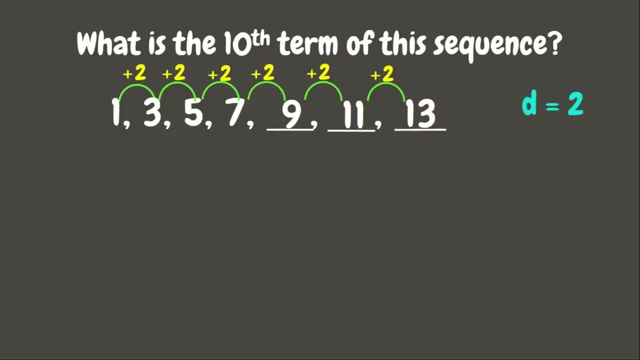 the common difference, which is two, and we already have the values of our terms. now let's just try to observe and look for some patterns in this sequence here, for the value of our first term, we have one. for the value of the second term, we can observe that we need to add. 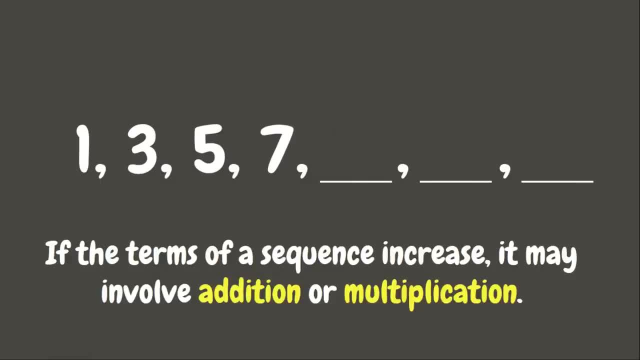 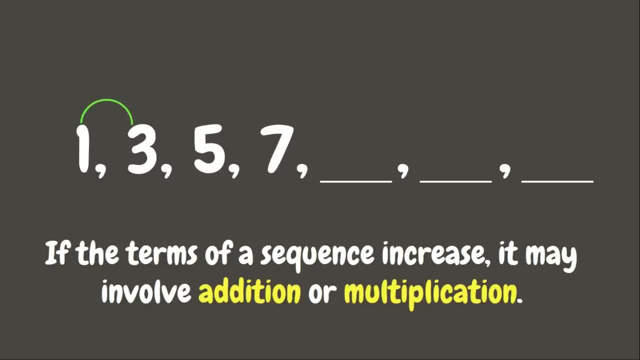 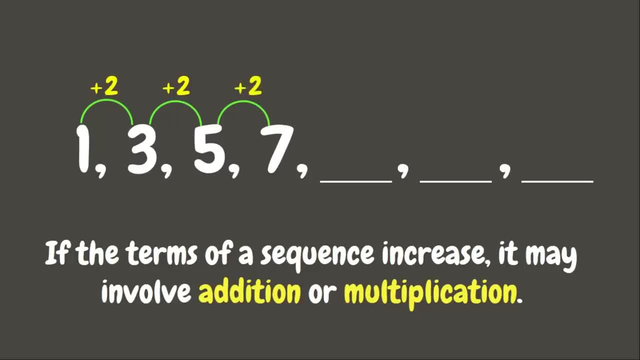 Next, 5 plus 2 is 7.. Therefore, if we add 2 to 7, we'll get the next term, which is 9.. And 9 plus 2 is 11.. And 9 plus 2 is 11.. 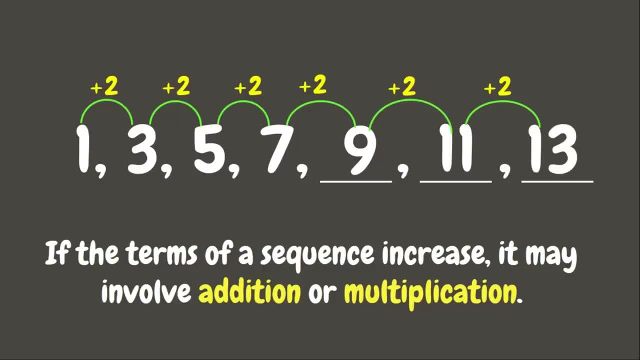 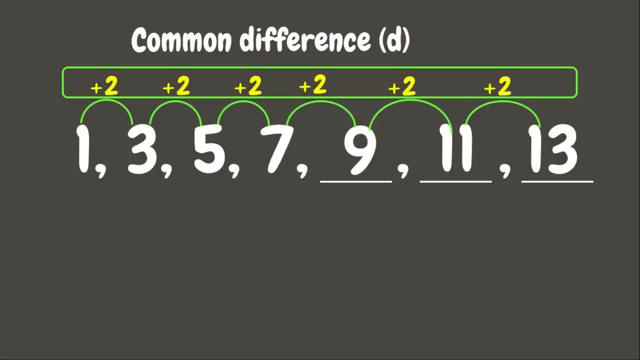 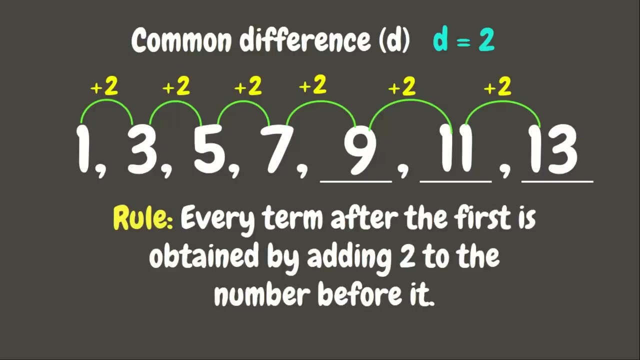 And 9 plus 2 is 11.. and then 13.. these numbers are what we call the common difference, which is represented by small letter d. this means that the common difference is 2.. here we can generate a general rule that for every term after the first is obtained by adding 2 to the number before it. 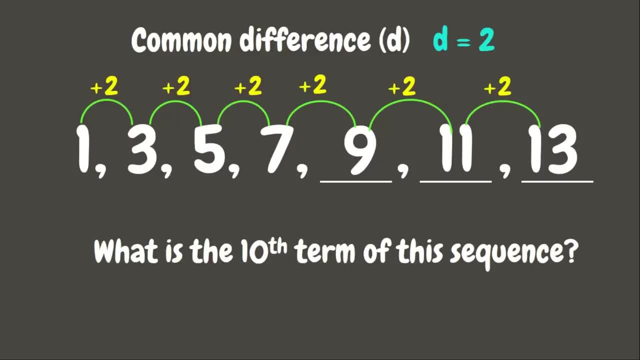 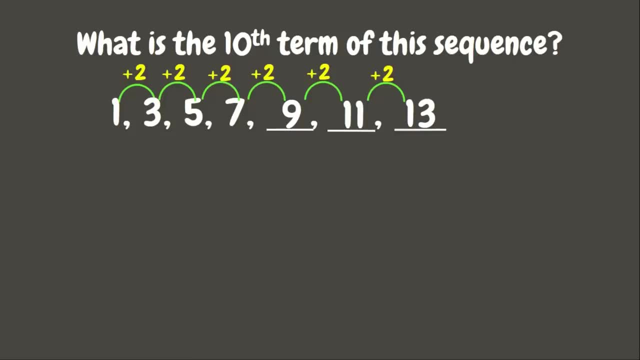 now, what if we are asked for the 10th term of this sequence? let's try and find out. we can try to determine the 10th term of this sequence by simply adding up 2 until we get the 10th term, but that would take us so much time. what if we are looking for the 50th term or the 100th term? are we? 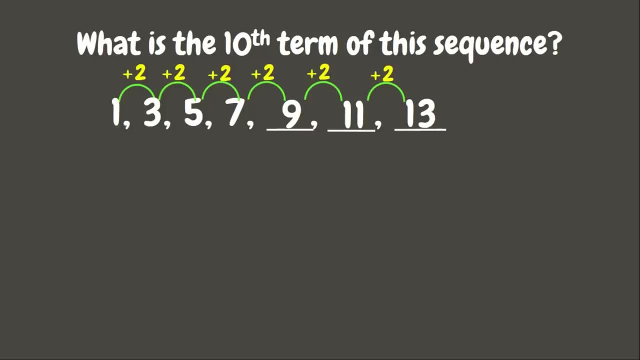 still going to add up 2 until we get them. now let us try to formulate an n-term rule for us to easily solve for any of the following questions: N- G- probable. then let's try to observe and look for some patterns in this sequence here. for the value of our first term, we have 1.. for the value of the second term, we can: 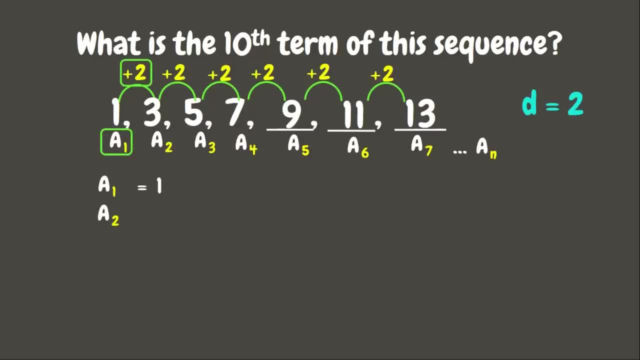 observe that we need to add 2 to our first term, which is 18 of 1.. and how many? 2 is our first theory. we can observe that we need to add 2 to our first term. which times did we add two? We add one time, So that would give us a sub one plus two times one. Now, 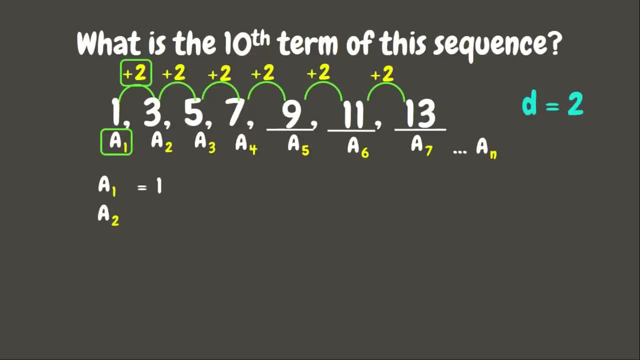 two to our first term, which is a sub one. and how many times did we add two? we add one time, so that would give us a sub one plus two times one. now for our third term, we can see that we added two to the first term two times, so that is a sub one plus two. 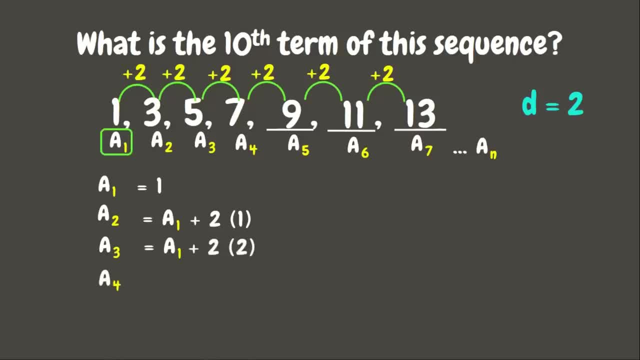 times two. now for our fourth term. we can see that we added three times of two to the first term, so that is a sub one plus two times three. we can see that we didn't add two to get our first term, which is one. now we can say that a sub one is equals to a sub one plus two times. 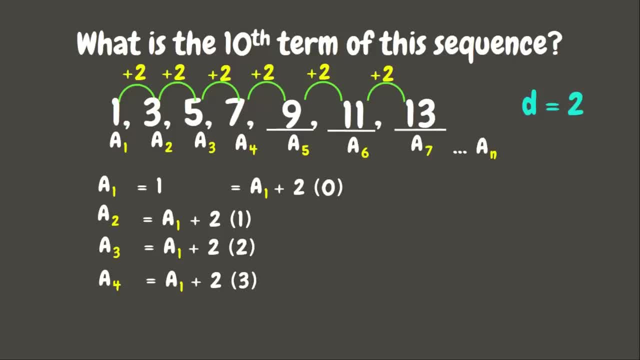 zero. now let us try to formulate a rule. by simple looking at some pattern here we can see that if we subtract one here, we'll get the number of times we add two. therefore, we can generate our formula as a sub one plus two, which is the common difference. 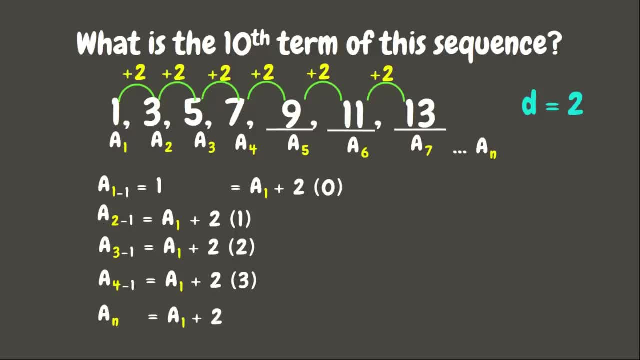 which is letter d times n minus one. now, this is our answer rule for this sequence. now let us try to get the 10th term of this sequence using this rule. since we are looking for the pamldigt term, that means we are looking for the answer of our tenth term. so let us now look for a. 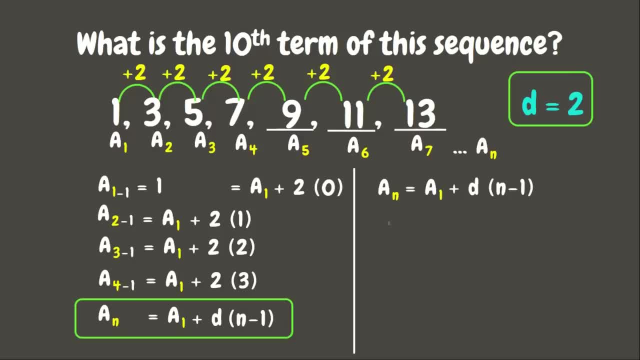 mustnah item. now let's look for our number of hands from ourنتemcom. now let's add two to our tenth term and then we'll see that we have this letter and plus two to be absent are looking for the. a sub 10 equals a sub 1, which is our first term: 1 plus the common difference. 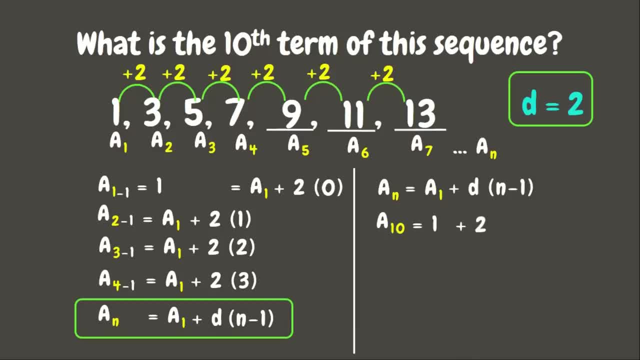 which is 2 times n minus 1. so here the value of our n is 10, since we are looking for the 10th term. so that gives us 10 minus 1. at this point, since we have two or more operations, we are going. 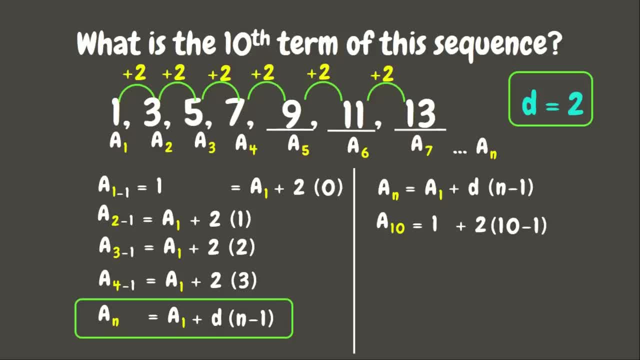 to apply the jeb, this rule. since we have grouping symbols, let us solve them first: 10 minus 1 is 9. next one is multiplication: 2 times 9 is 18, and now we have our last operation, which is addition. so that is, 1 plus 18 is 19. therefore, the 10th term of this sequence is: 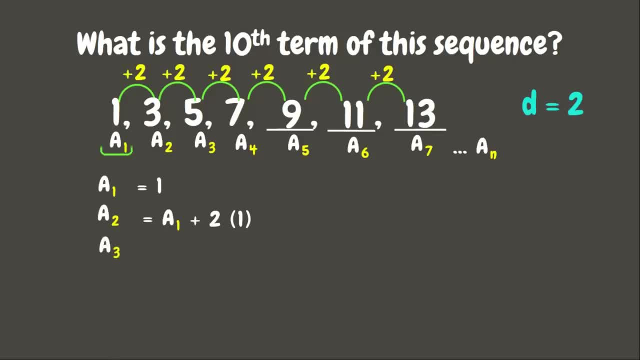 for our third term, we can see that we added two to the first term two times, So that is a sub one plus two times two. Now for our fourth term, we can see that we added three times of two to the first term, So that is a sub one plus two times three. We can see that we didn't add two to get. 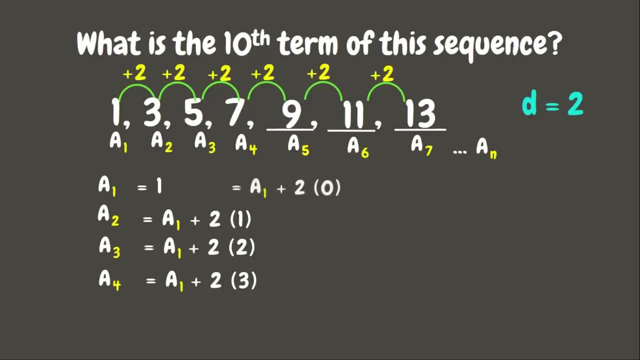 our first term, which is one. Now we can say that a sub one is equal to a sub one plus two times zero. Now let us try to formulate a rule. by simply looking at some pattern Here we can see that if we subtract one here, we'll get the number of times we add two. 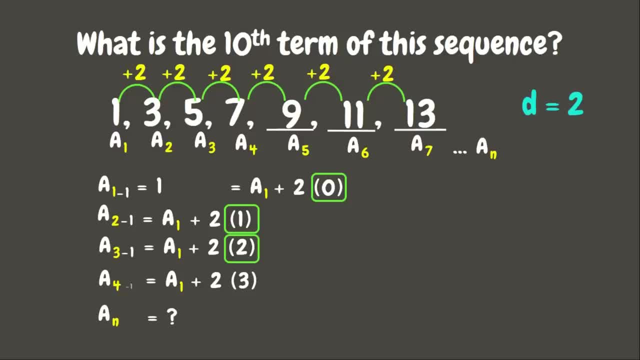 Therefore, we can generate our formula as a sub: one plus two, which is the common difference, which is letter d times n minus one. Now, this is our n-term rule for this sequence. Now let us try to get the tenth term of this sequence using this rule, Since we are looking for the tenth term. 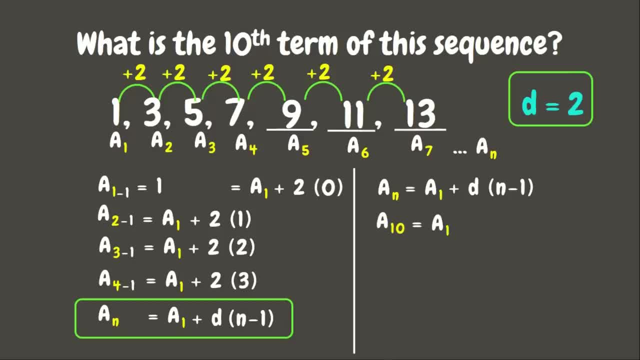 that means we are looking for the. a sub tenth Equals a sub one, which is our first term. one plus the common difference, which is two times n minus one. So here the value of our n is ten, since we are looking for the tenth term. So that gives us ten minus one At this point. 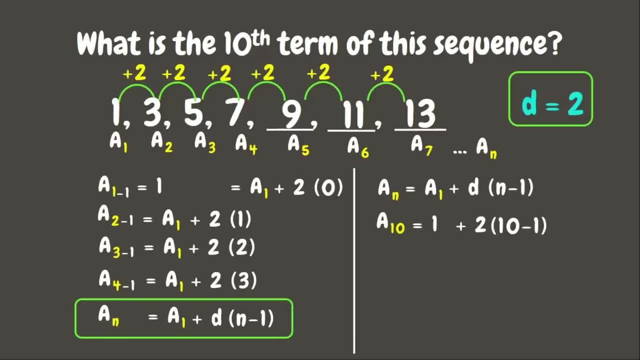 since we have two or more operations, we are going to apply the Jambla's rule. Since we have, let us solve them first. Ten minus one is nine. Next one is multiplication: Two times nine is eighteen. And now we have our last operation, which is addition. So that is one plus eighteen. 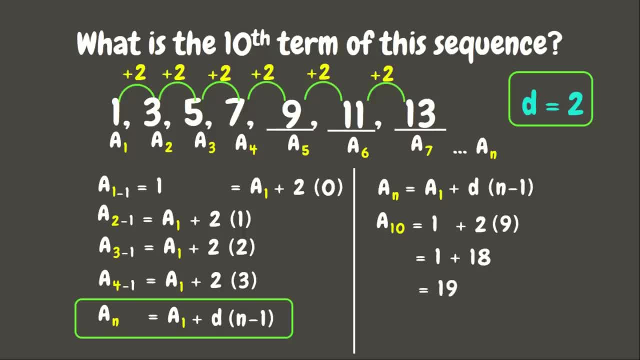 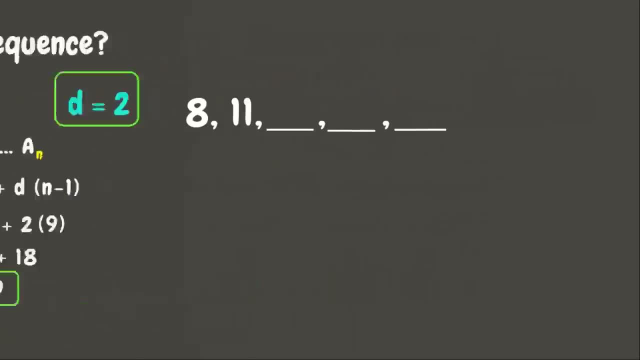 is nineteen. Therefore the tenth term of this sequence is nineteen. Great job. Now let's have another example. So this time we have the sequence two, five, eight and eleven. Here we can see that if we add three to each term, we'll get the next term. So two plus three is five plus three is eight. 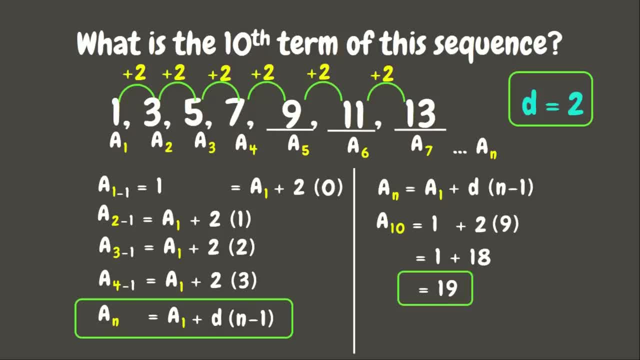 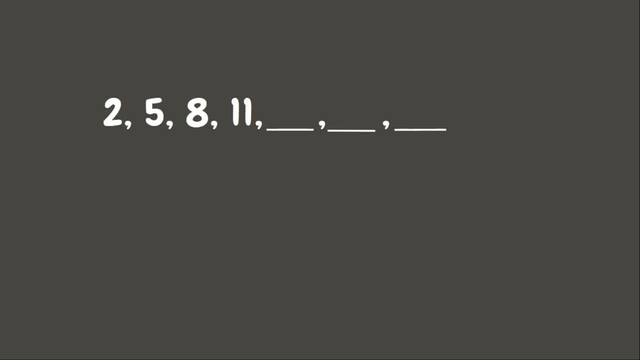 19. great job. now let's have another example. This time we have the sequence 2, 5,, 8, and 11.. Here we can see that if we add 3 to each term, we'll get the next term. So 2 plus 3 is 5, plus 3 is 8, plus 3 is 11.. Now 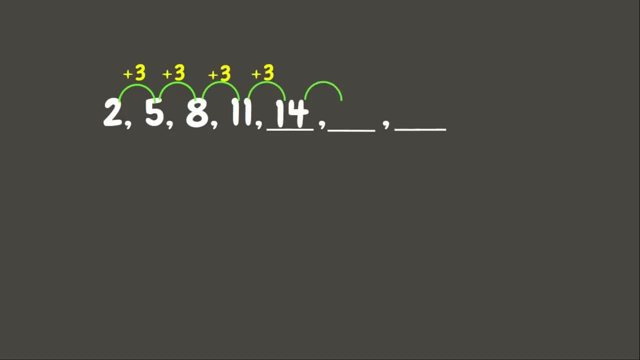 the next term would be 14,, 17, and 20.. Here we can see that we have the common difference, which is 3.. Since this sequence have common difference, we can use our n-term rule that we used earlier to get the 17th term. Again, our n-term rule is: 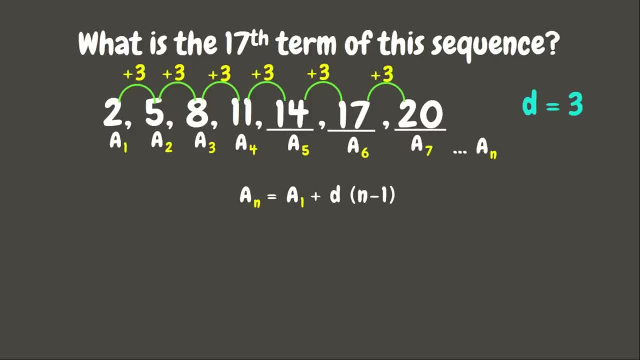 14,, 17, and 20.. So we have 8 sub 17 equals 8 sub 1 plus 3 times n minus 1.. Since we are looking for the 17th term, we have 8 sub 17 equals 8 sub 1, or the first term, which is 2 plus the. 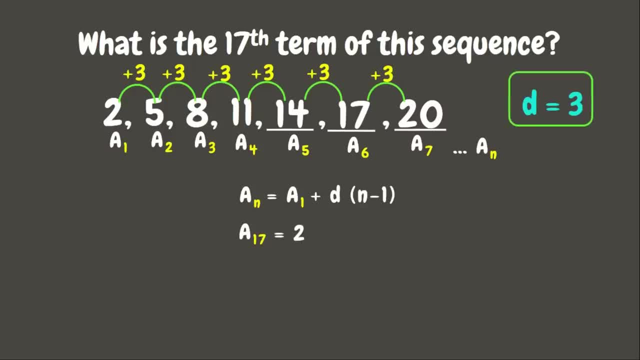 common difference, which is 3 times n minus 1.. Here, our n-term that we are looking for is 17.. Therefore, that is 17 minus 1.. Again, at this point we are going to use the jamdest rule. 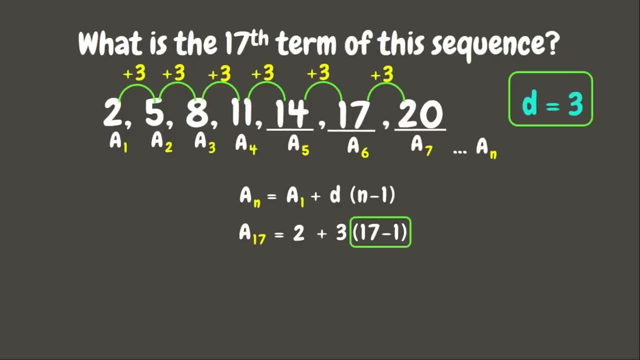 Since we have grouping symbols, let us solve them first: 17 minus 1 is 16.. Next is multiplication 3 times 16 is very good, It's 48.. Lastly, we have 2 plus 48, which is 50. And now that is our 17th term. 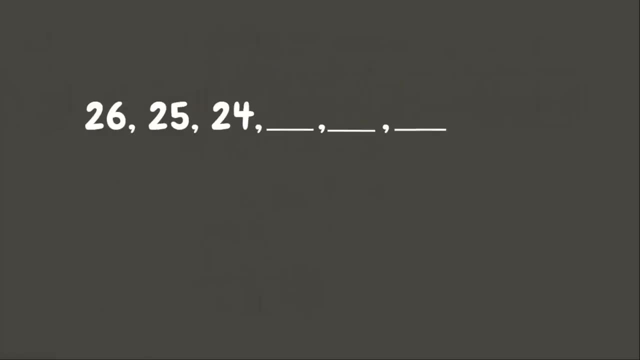 Wonderful. Well, let's have another example. This time we have 26,, 25,, 24.. As you can see, the sequence is decreasing. Therefore, it may involve subtraction or division. Now let us try What should. 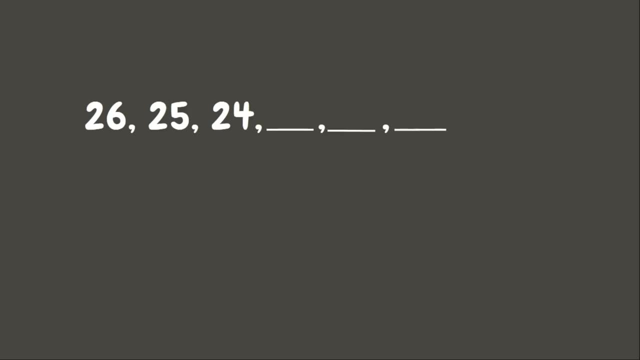 we do to 26 to get the next term, which is 25? Great job. We are going to subtract 1.. So 26 minus 1 is 25.. And then we are going to subtract 1.. And then we are going to subtract. 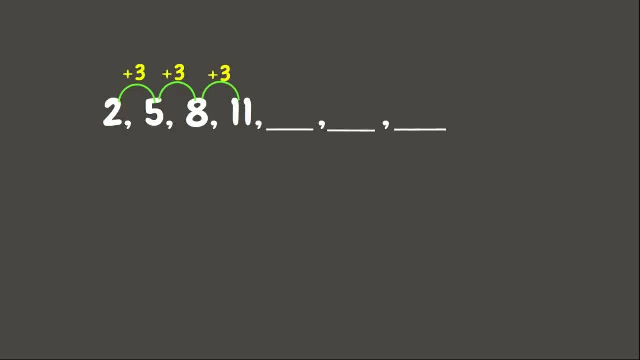 plus three is eleven. Now the next term would be fourteen, seventeen and twenty. Here we can see that We have the common difference, which is 3.. Since this sequence have common difference, we can use our n-term rule that we used earlier to get the 17th term. 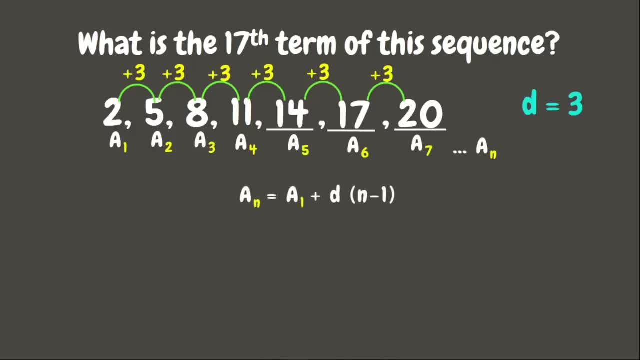 Again, our n-term rule is: a sub n equals a sub 1 plus 3 times n minus 1.. Since we are looking for the 17th term, we have a sub 17 equals a sub 1, or the first term, which is 2 plus the common difference, which is 3 times n minus 1.. 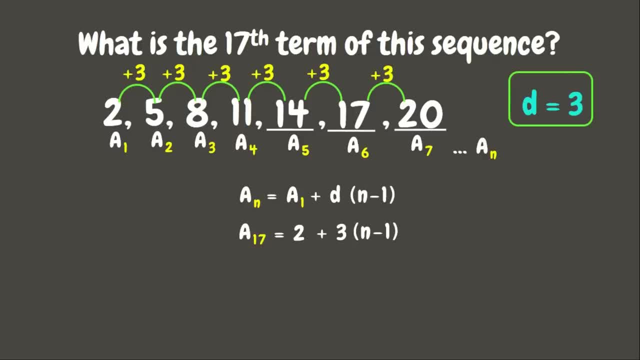 Here, our n-term that we are looking is 17.. Therefore, that is 17 minus 1.. Again, At this point we are going to use the Jambliss rule. Since we have grouping symbols, let us solve them first. 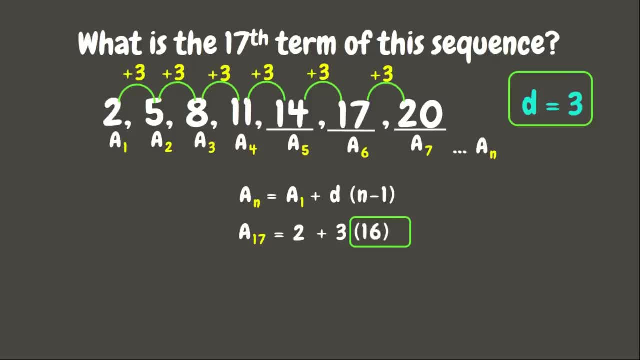 17 minus 1 is 16.. Next is multiplication 3 times 16 is very good, It's 48.. Lastly, we have 2 plus 48, which is 50. And now that is our 17th term. 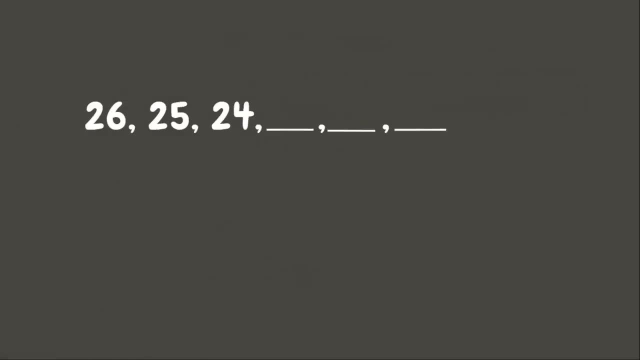 Wonderful. Let's have another example. This time we have 26,, 25,, 24.. As you can see, the sequence is decreasing. Therefore, it may involve subtraction or division. Now let us try. What should we do to 26 to get the next term, which is 25?? 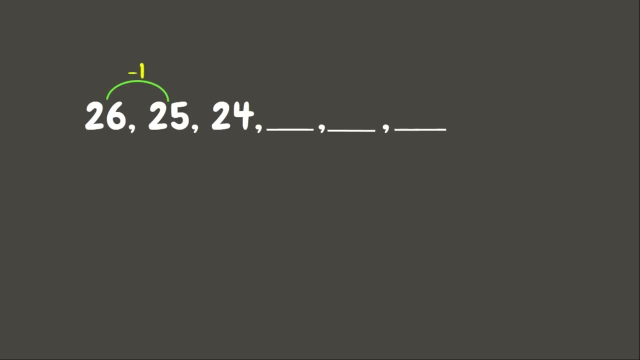 Great job. We are going to subtract 1.. So 26 minus 1 is 25.. Minus 1 is 24.. Minus 1 is 23.. Next is 22.. And lastly, we have 21.. 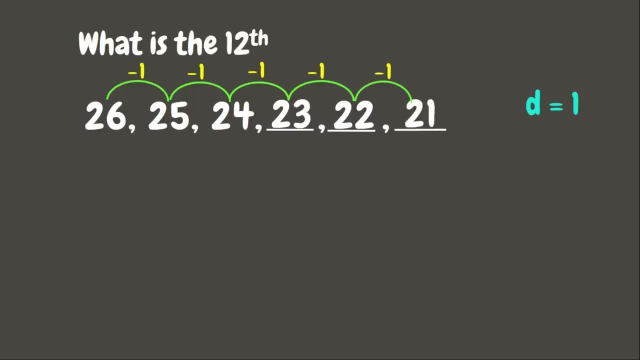 Therefore, our common difference is 1.. Now what is the 12th term of this sequence? Since they have common difference, we can still use the n-term rule that we used earlier. So that is, a sub n equals a sub 1 plus b times n minus 1.. 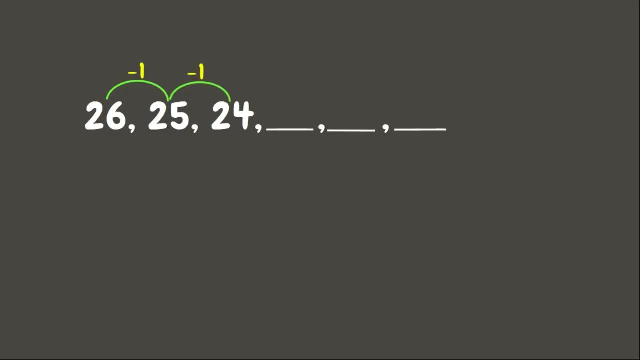 1.. And then we are going to subtract 1.. And then we are going to subtract 1.. And then 25 minus 1 is 24 minus 1 is 23, next is 22 and lastly we have 21. therefore our common difference. 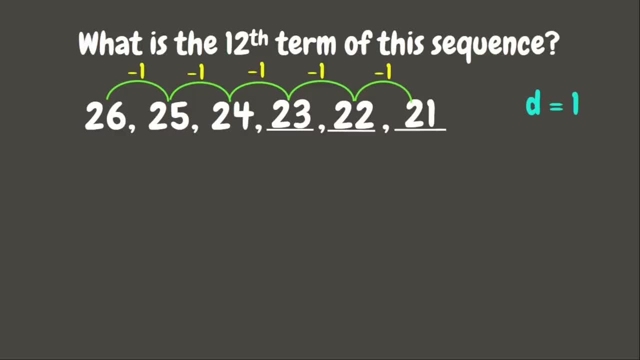 is 1.. now what is the 12th term of this sequence? since they have common difference, we can still use the n term rule that we used earlier. so that is, a sub n equals a sub 1 plus b times n minus 1. but since in this sequence, instead of adding we are subtracting, we are going to change this one as: 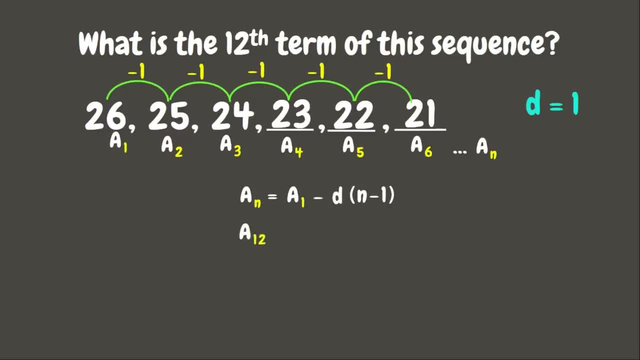 minus b. now let us solve: a sub 12 equals a sub 1, or the first term, which is 26 minus the common difference, which is 1 times n minus 1, which is 12 minus 1. let us use our gem, this rule. let's solve first the operation inside the grouping symbol, which is 12 minus 1. 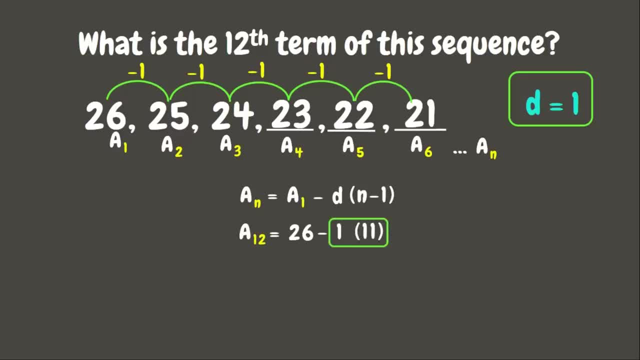 that is 11.. next is: we are going to multiply 11 times 1 is 11. and lastly, let us subtract 26 and 11 and the result is 15.. therefore, the 12 term of this sequence is 15.. wonderful. 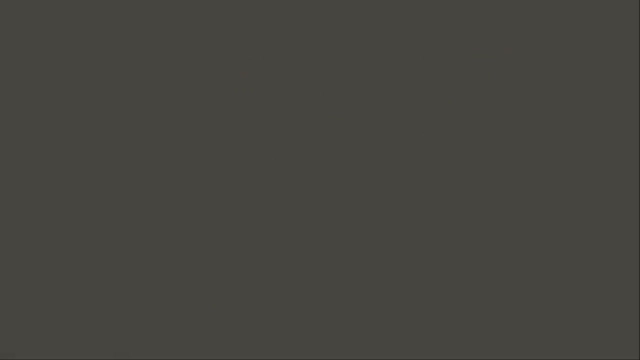 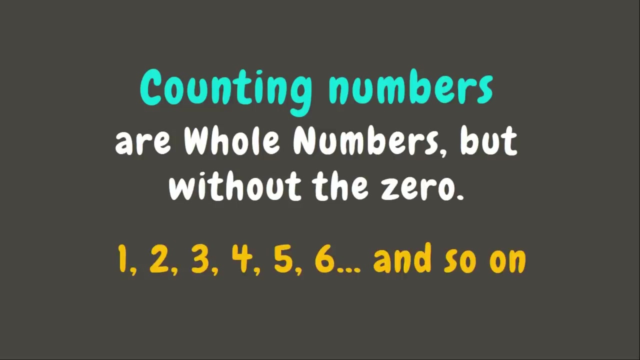 now there is another way of formulating an n-term rule. if the sequence doesn't have the common difference, we can use counting numbers. counting numbers are whole numbers, but without zero. so that is one, two, three, four, five, six and so on. now let's try an example. we have here a sequence. 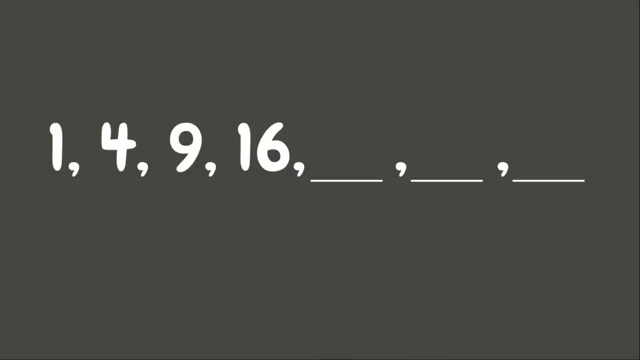 one, four, nine and sixteen, and the next three terms are missing. so if a sequence doesn't have a common difference, we can use the counting numbers. here we're just simply going to count the number of terms we have in this sequence. we have one, two, three, four, five, six, seven and so on. 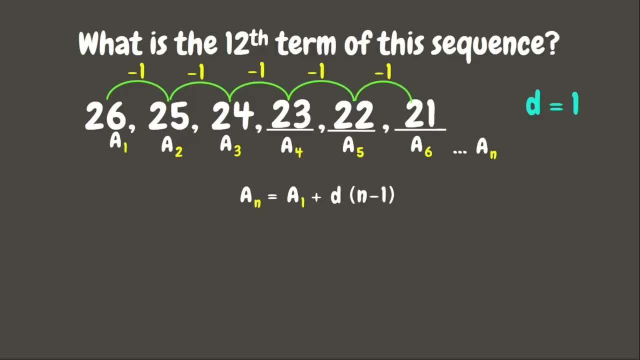 But since, in this sequence, instead of adding we are subtracting, We are going to change this one as minus b. Now let us solve: a sub 12 equals a sub 1, or the first term, which is 26.. 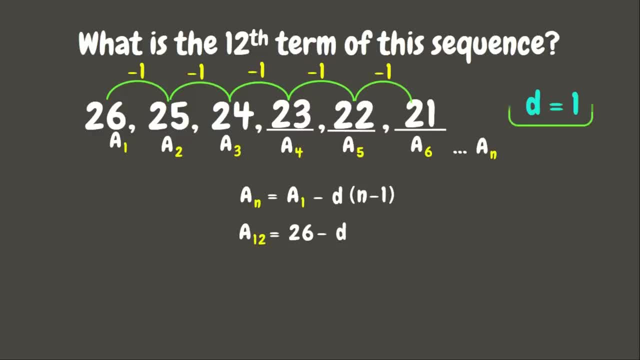 Minus the common difference, which is 1.. Times n minus 1, which is 12 minus 1.. Let us use our gem list rule. Let's solve first the operation inside the grouping symbol, Which is 12 minus 1.. 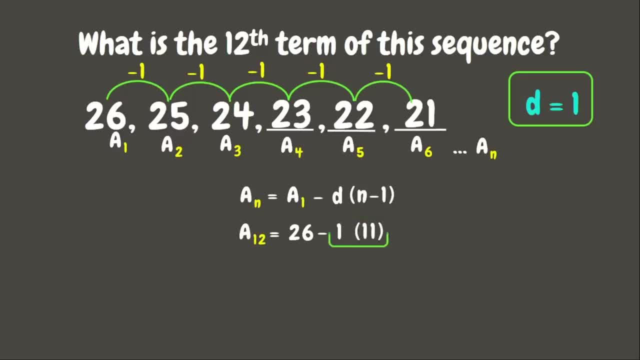 That is 11.. Next is: we are going to multiply 11 times 1 is 11.. And lastly, let us subtract 26 and 11.. And that gives us 15.. Therefore, the 12th term of this sequence is 15.. 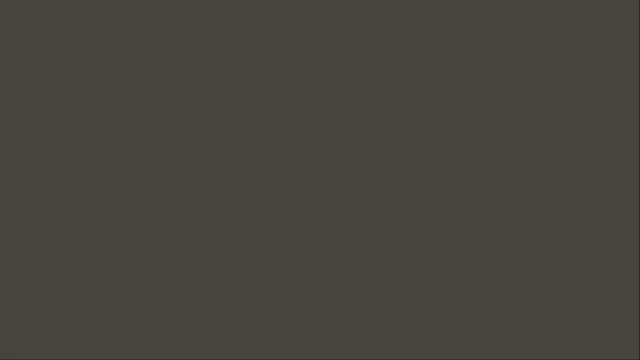 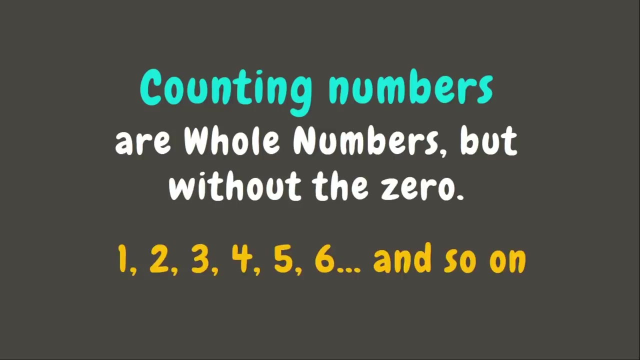 Wonderful. Now there is another way of formulating an n-term rule. If a sequence doesn't have the common difference, we can use counting numbers. Counting numbers are whole numbers, but without zero. So that is 1,, 2,, 3,, 4,, 5,, 6, and so on. 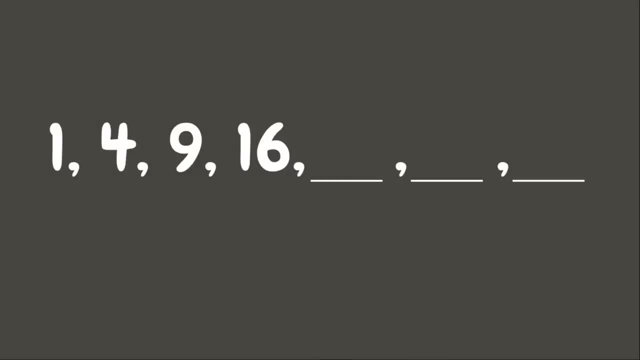 Now let's try an example. We have here a sequence 1,, 4,, 9, and 16. And the next three terms are missing. So if a sequence doesn't have a common difference, we can use the counting numbers. 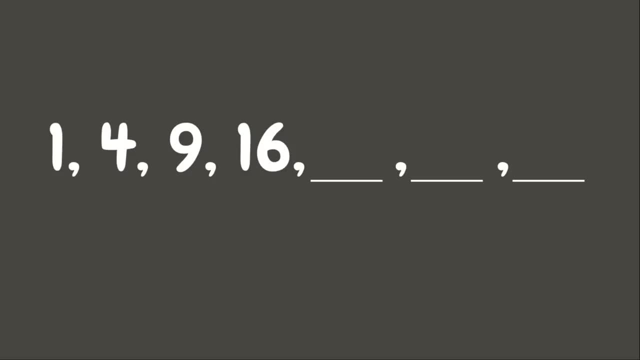 Here we are just simply going to count the number of terms We have in this sequence. We have 1,, 2,, 3,, 4,, 5,, 6,, 7, and so on, Which is the n-term? 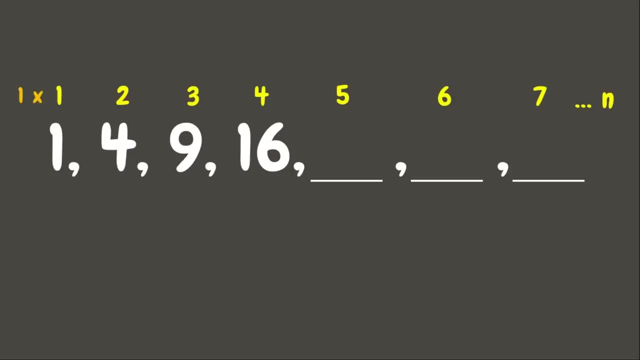 Here we can see that if we multiply 1 to 1,, we'll get the value of our first term, which is 1.. If we multiply 2 to 2,, we'll get the value of our second term, which is 4.. 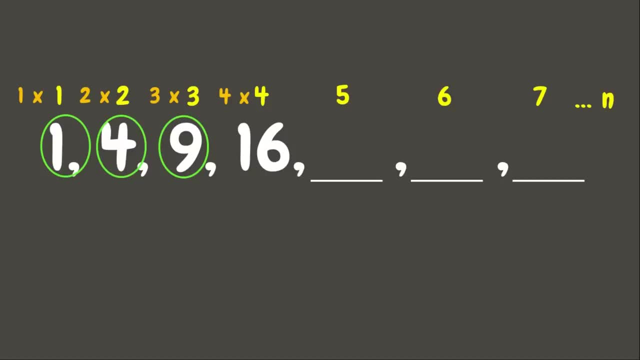 And then 3 times 3 is 9.. 4 times 4 is 16.. Here we can see that we have a common difference. We can see a pattern. So let us try: 5 times 5, we'll get 25.. 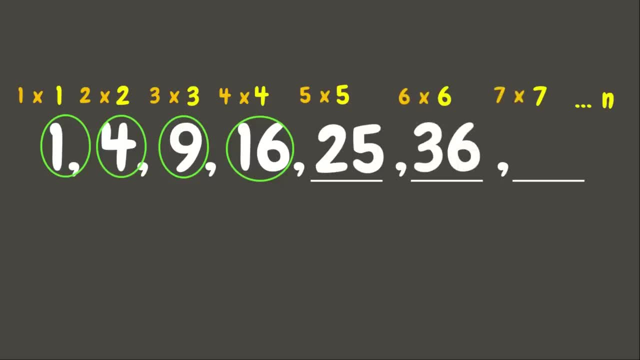 6 times 6, 36.. 7 times 7 is 49. And to get our n-term we can say n times n. Now we can see that if we multiply the counting number by itself or squaring counting numbers, 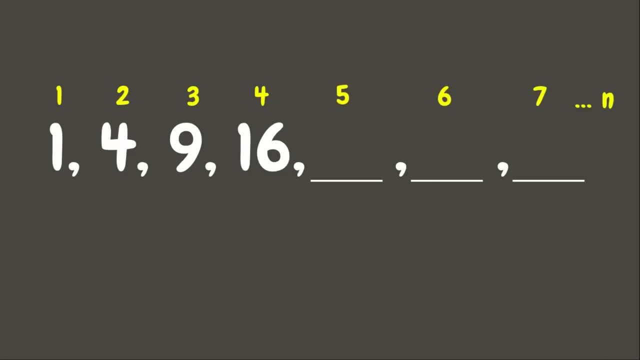 which is the enter. here we can see that if we multiply one to one, we'll get the value of our first term, which is one. if we multiply two to two, we'll get the value of our second term, which is four. and then, three times three is nine, four times four is sixteen. here we can see a pattern. so let 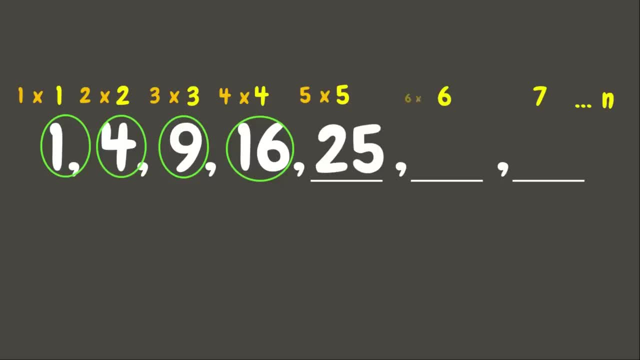 us try: five times five, we'll get 25, 6 times 6, 36. 7 times 7 is 49 and to get our n term we can say n times n. now can see that if we multiply the counting number by itself or squaring counting numbers, 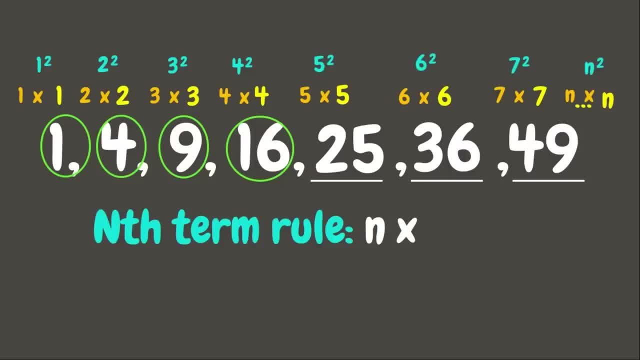 we'll get the value of each term. therefore, our n term rule here is n times n or n squared. so if you're looking for the 10 term, that is 10 times 10 and we'll get 100, and if we are looking for the 9 term, that means 9 times 9, which is 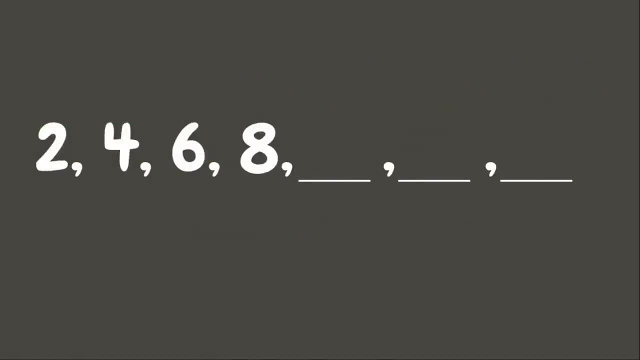 1. great job. now let's have another example. first time we have two, four, six, eight. now let's just try to solve this using counting numbers. here we can observe a pattern that if we multiply two to the counting numbers, we'll get the value of each term. for example, we have two times one, we'll 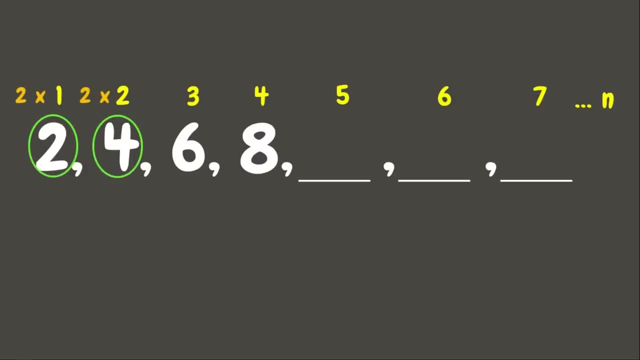 get our first break. discuss two, two times two. we have four. two times three. we have six. two times four, we have eight. therefore, for our fifth term, we can multiply two to five. that is ten. two times six is twelve and two times the seventh term, which is forty. therefore, for us to get the n term that 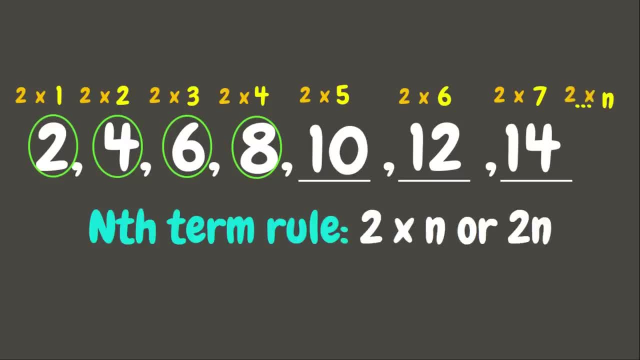 is two times n. therefore, our n term rule here is two times n or two n. so if we are looking for the 10 term, that is 2 times 10, which is 20.. and if you're looking for the 17 term, that is 2 times 17. 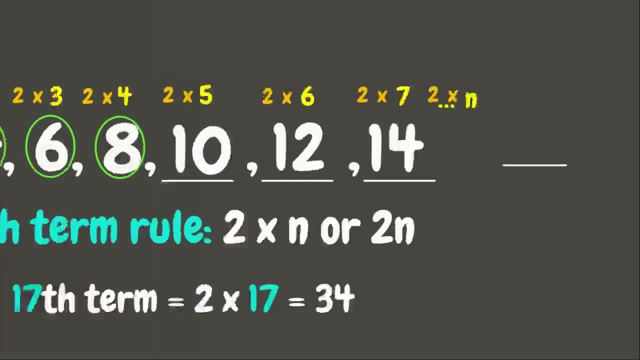 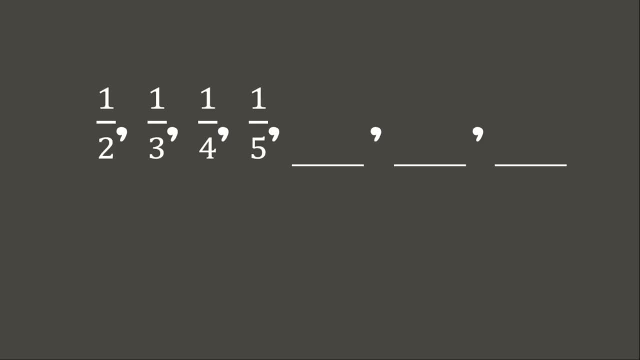 which is 34.. awesome, let's have another example. this time, let us try it with fractions. here we have the sequence: one half, one third, one fourth, one fifth. what do you think are the next three terms? now, let us try to solve this using our counting numbers, which represent the order of the 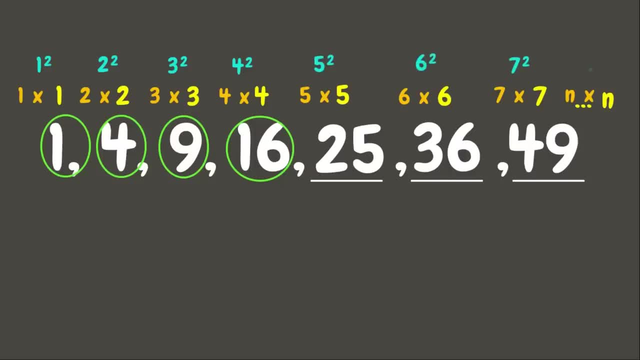 we'll get the value of each term. Therefore, our n-term rule here is n times n or n squared. So if you're looking for the 10-term, that is 10 times 10, and we'll get 100.. 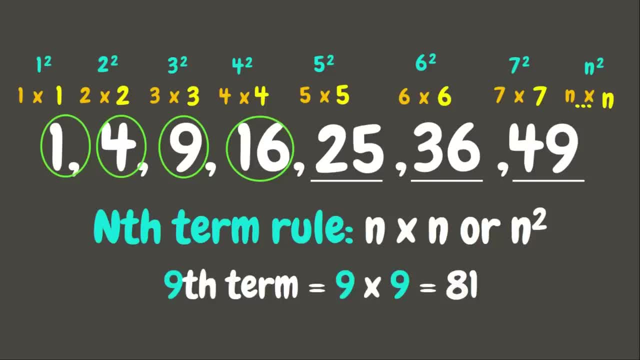 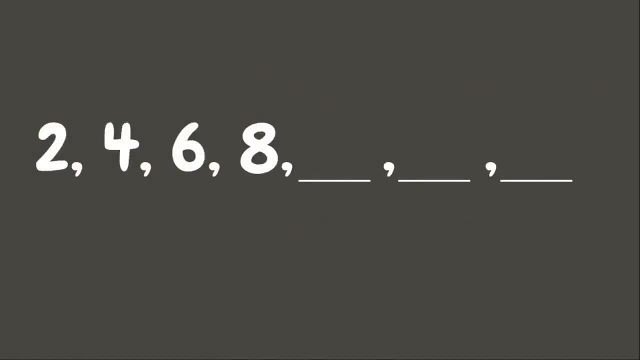 And if you're looking for the 9-term, that means 9 times 9,, which is 81.. Great job. Now let's have another example. This time we have 2,, 4,, 6,, 8.. 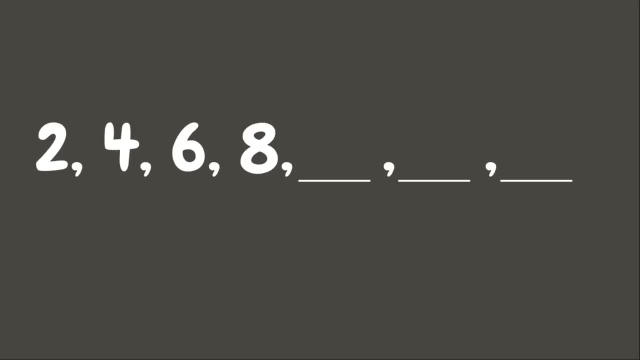 Now let's just try to solve this using counting numbers. Here we can observe a pattern: that if we multiply 2 to the counting numbers, we'll get the value of each term. For example, we have 2 times 1, we'll get our first term, which is 2.. 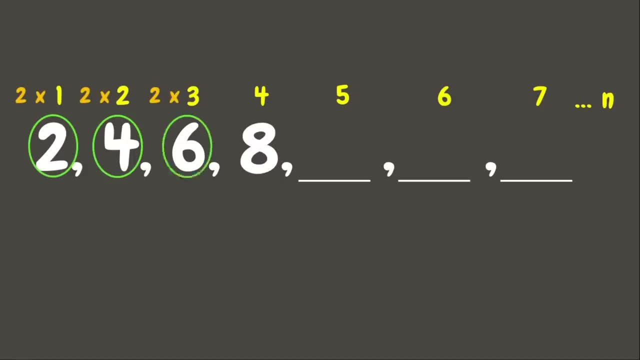 2 times 2,, we have 4.. 2 times 3,, we have 6.. 2 times 4,, we have 8.. Therefore, for our 5th term, we can multiply 2 to 5.. 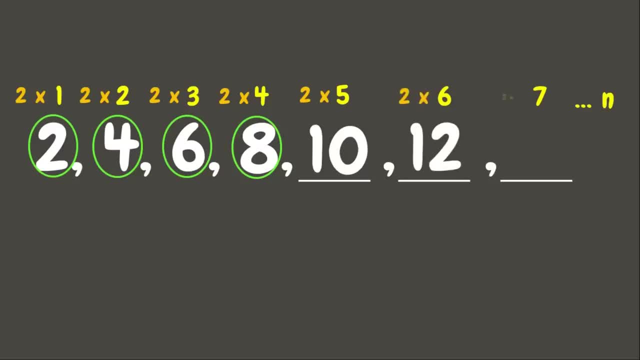 That is 10.. 2 times 6 is 12. And 2 times the 7th term, which is 14.. Therefore, for us to get at the n-term, that is 2 times n. Therefore, our n-term rule here is 2 times n or 2n. So 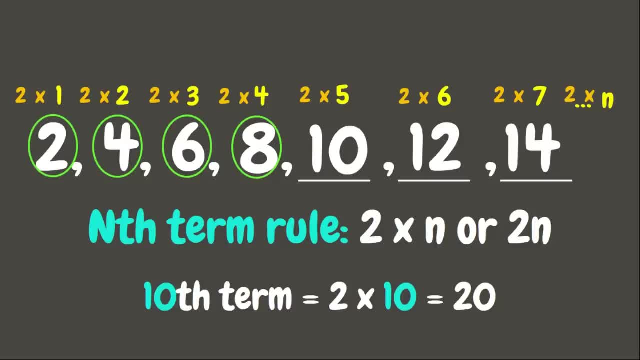 if we are looking for the 10-term, that is 2 times 10,, which is 20.. And if we are looking for the 17-term, that is 2 times 17,, which is 34.. Awesome, Let's have another example. 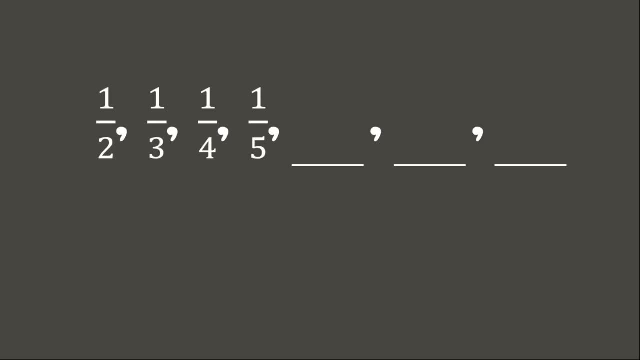 So next time let us try it with fractions. Here we have the sequence: 1 half, 1 third, 1 fourth, 1 fifth. What do you think are the next three terms? Now let us try to solve this. 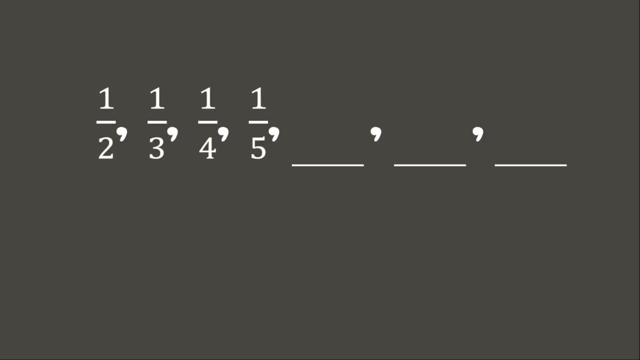 using our counting numbers, which represent the order of the terms Here, we can see that if we add 1 to the counting numbers, we'll get the denominator. So we have 1 plus 1.. We'll get the denominator of our first. 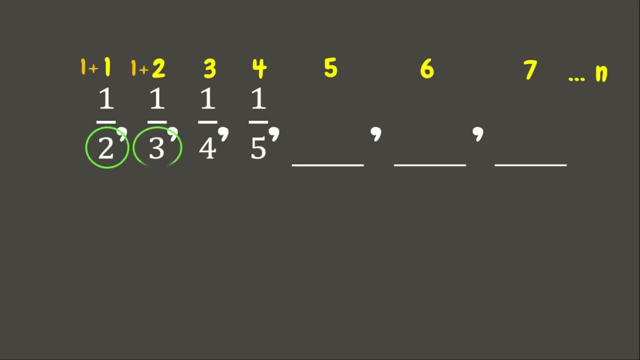 term. So let's try it with fractions. Here we have the sequence 1 half, 1 third, 1 fourth, which is 2.. Therefore, our fifth term would be 1. sixth. For our sixth term, we have 1.